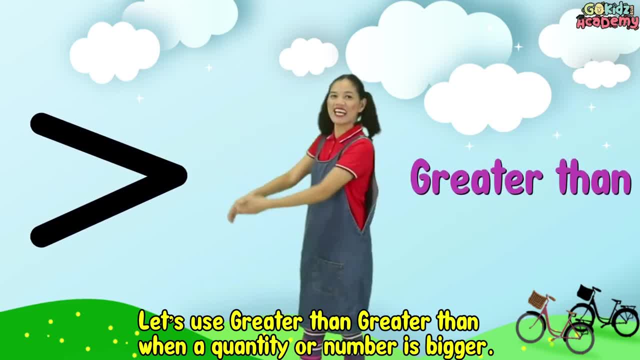 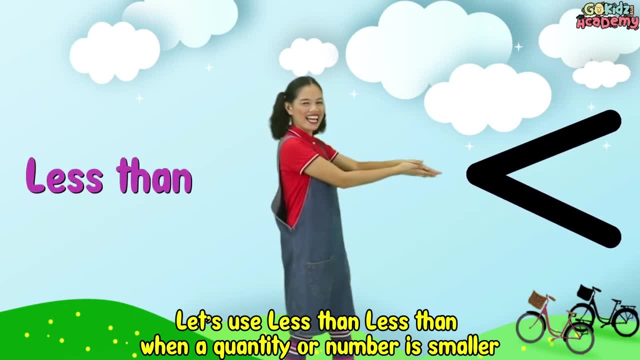 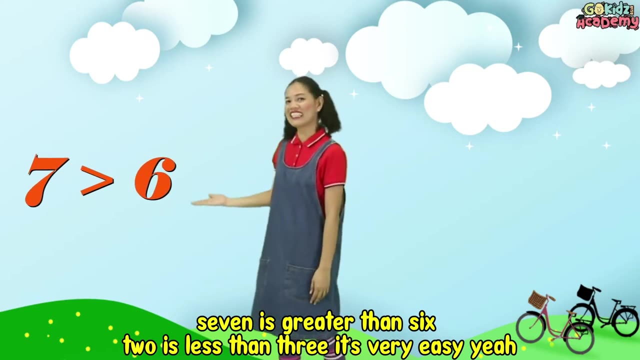 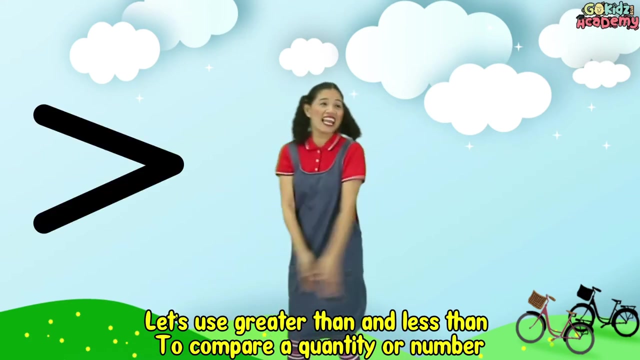 Let's use greater than greater than When the quantity or number is bigger. Let's use lesser than less than When the quantity or number is smaller. Seven is greater than six. Two is less than three. It's very easy. yeah, Let's use greater than and less than. 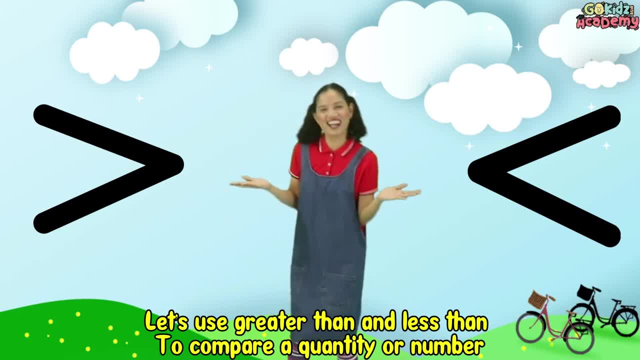 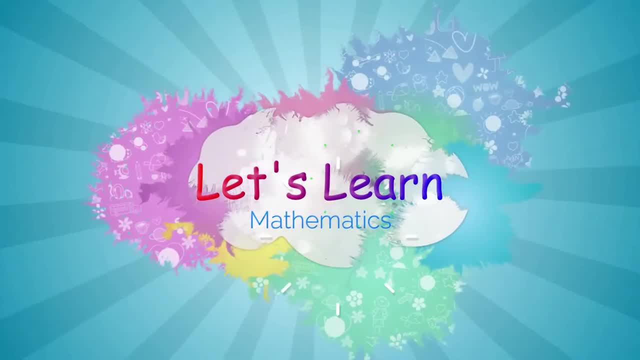 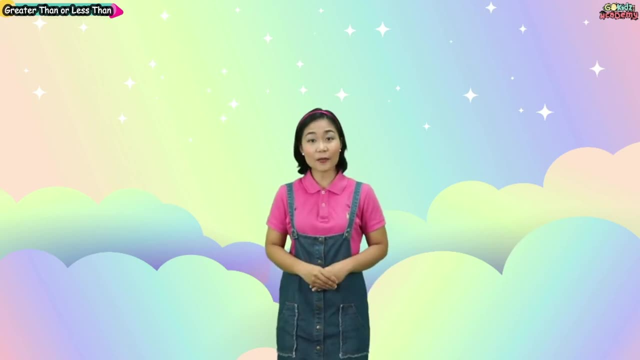 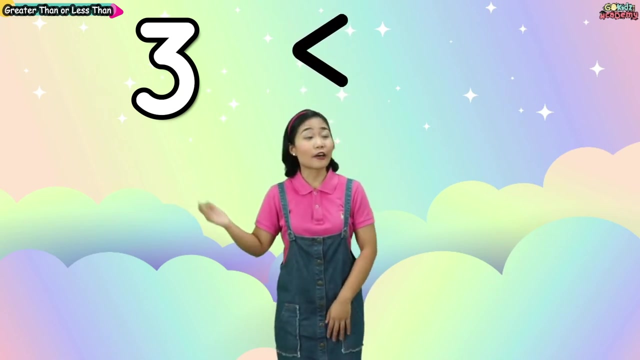 To compare a quantity or a number. Today we have a new lesson, And it's all about greater than and less than. We use greater than if the first number is bigger or greater than the second number, And we use lesser than And less than if the first number is smaller than the second number. 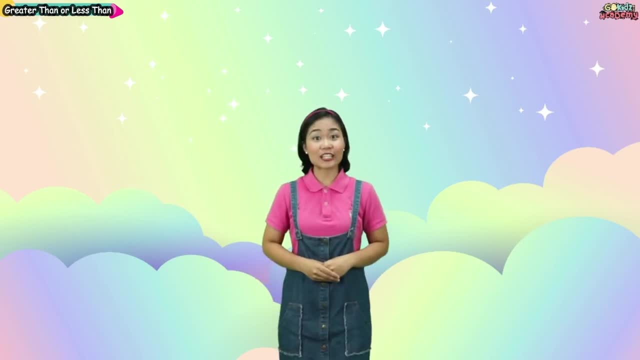 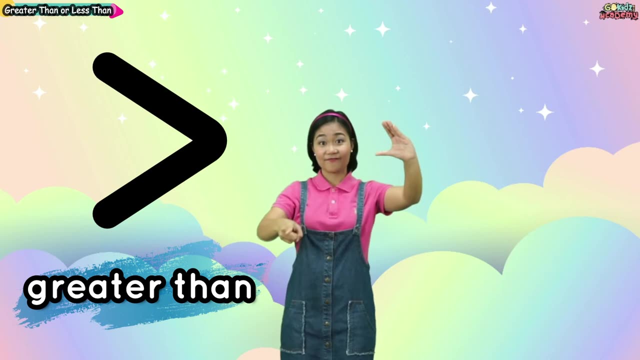 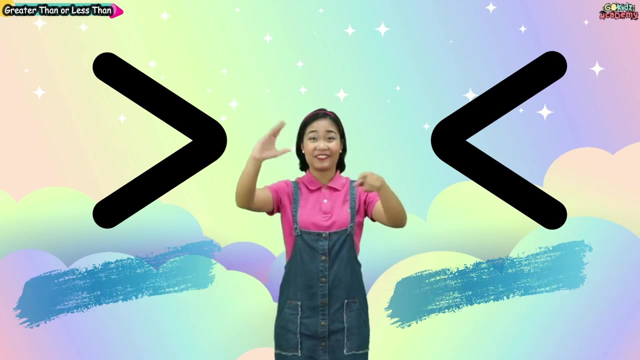 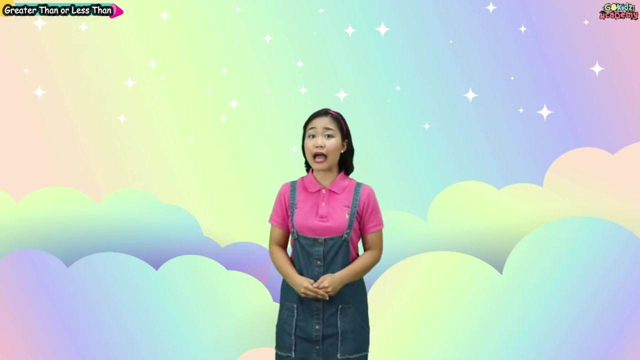 So that you can easily remember. Let's learn their symbols: Greater than is like this And less than is like this. Okay, did you get it? I have here A few examples of greater than and less than. Can you see I have fruits on my both sides. 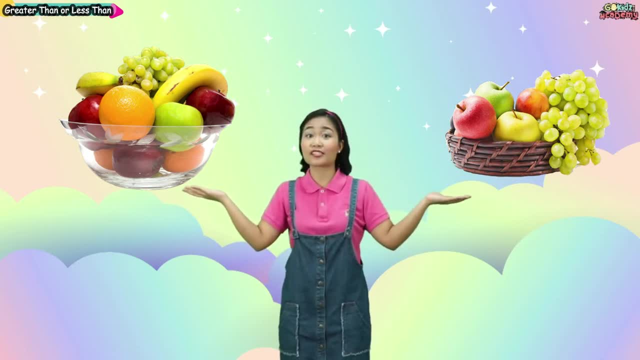 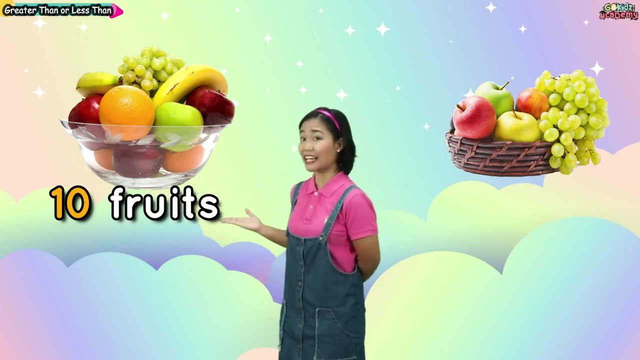 And let's try to count how many fruits are on this side: One, two, three, four, five, six, seven, eight, nine, ten fruits on this side. And let's try to count on this side. There are ten fruits on this side. 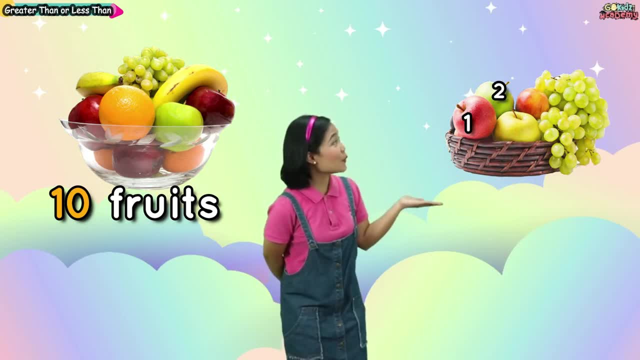 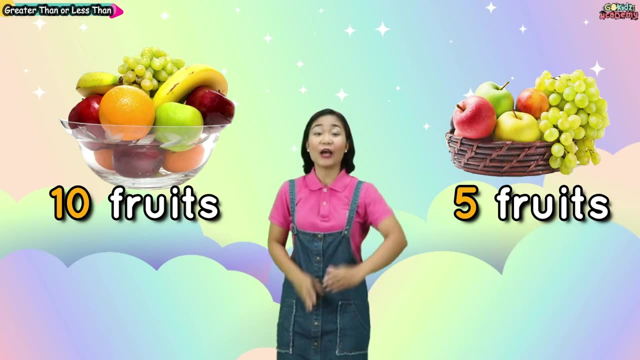 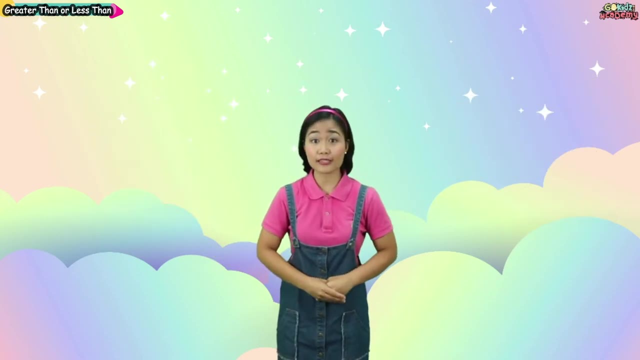 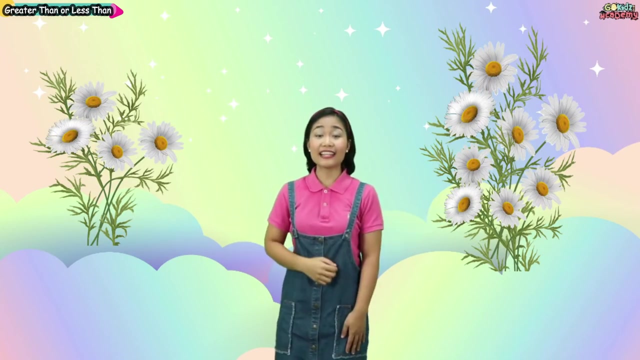 There are one, two, three, four, five fruits on this side, So our answer should be: Greater than Ten is greater than five. Let's go to the next example. Oh, I have flowers on both sides. Let's count how many flowers are on this side. 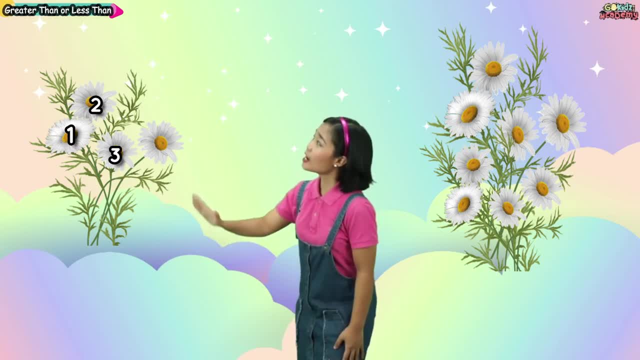 One, two, three, four, five, six, seven, eight, nine, ten fruits on this side: One, two, three, four photos. And let's count how many flowers are on this side. And let's count how many flowers are on this side. 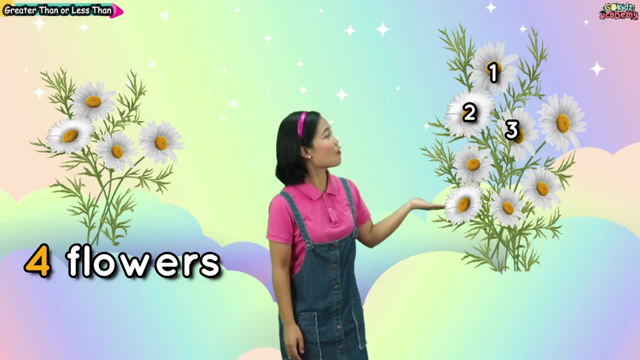 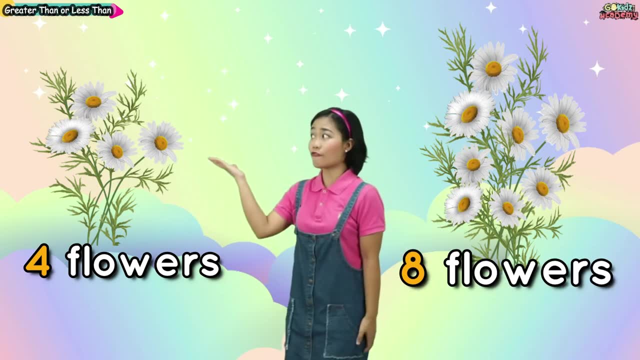 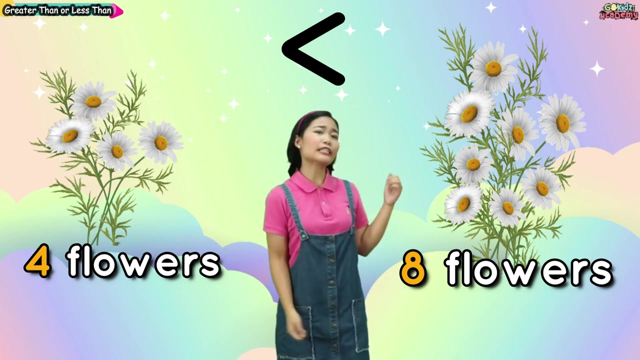 One, two, three, four, five, six, seven, eight, nine, ten fruits on this side. We have four on this side And we have eight flowers on this side. What should be our answer? Can I hear your answer? Very good, Our answer should be less than, because 4 is smaller than 8.. 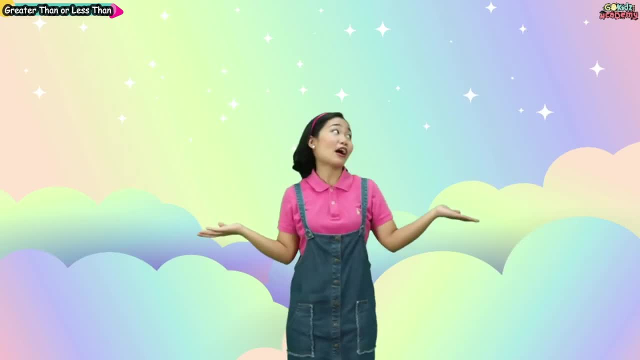 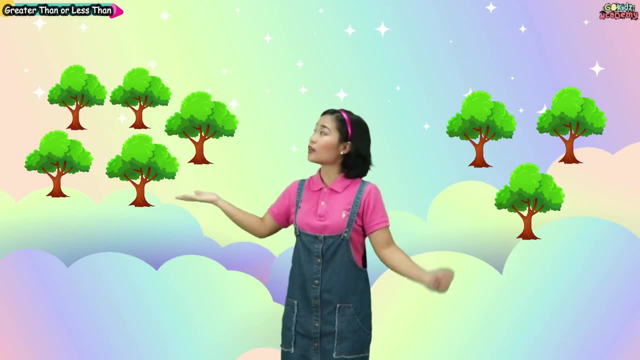 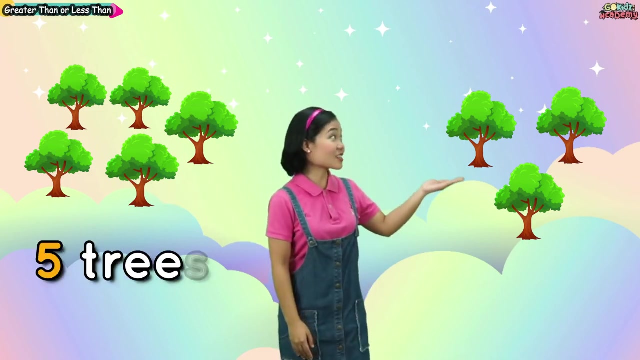 Now it's your turn. Oh, I have trees on both sides. Let's count first how many trees are on this side: 1,, 2,, 3,, 4, and 5.. Let's go on this side. 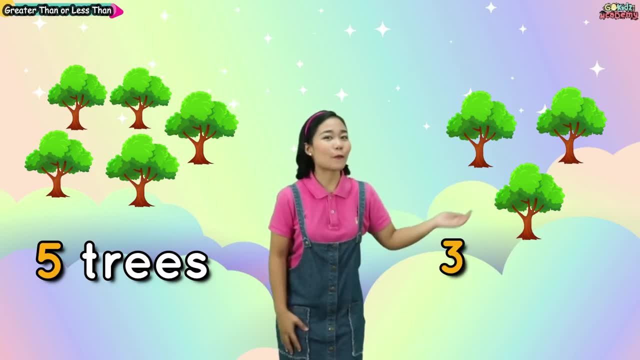 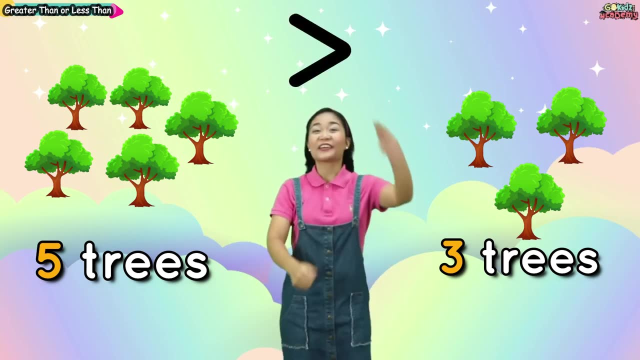 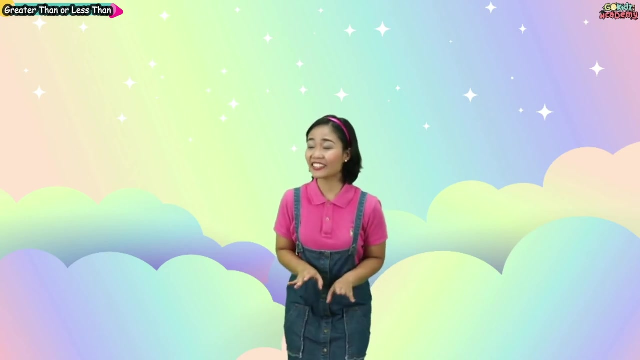 1, 2, 3.. What should be our answer? Very good, Our answer is greater than, because 5 trees are more than 3 trees. Next one: Oh, do you see what I see? There is one chicken here. 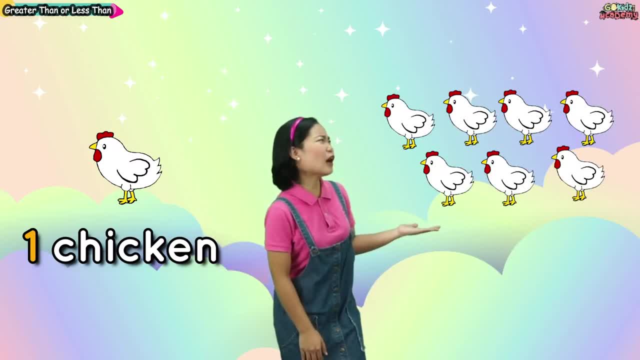 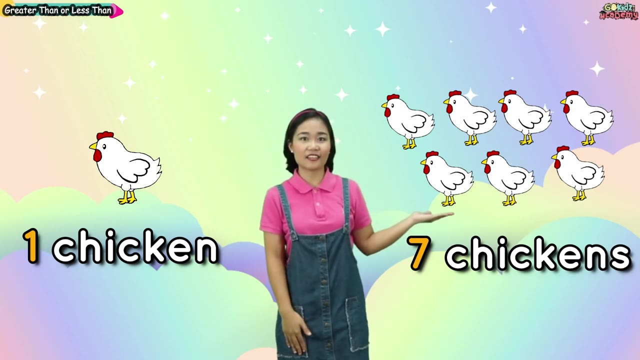 And there are. let's count how many chickens are these? 1,, 2,, 3,, 4,, 5,, 6, 7 chickens are on this side. So what should be our answer? It is less than. 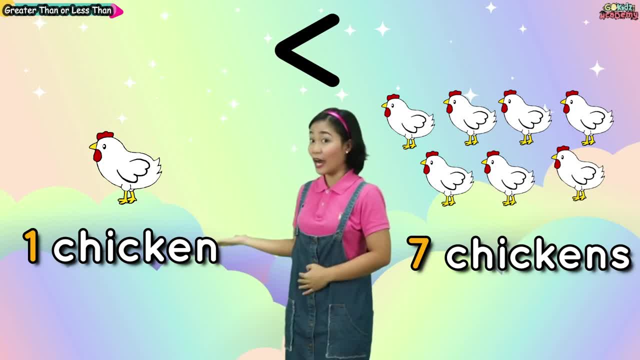 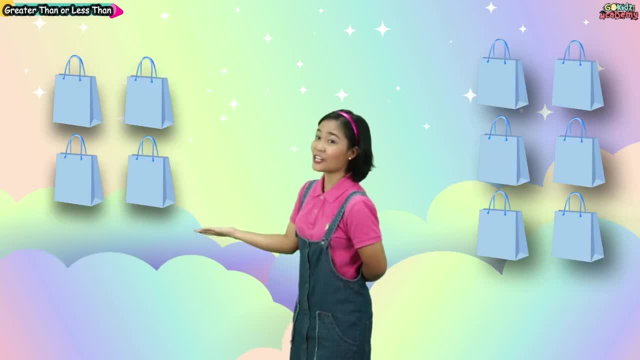 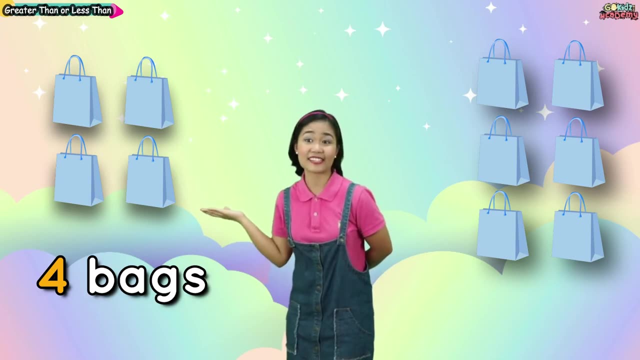 Less than, because 1 is smaller, Less than 7, of course, Let's count how many banks are here: 1,, 2,, 3,, 4.. We have 4 banks. And how about on this side? 1,, 2,, 3,, 4,, 5,, 6 banks? 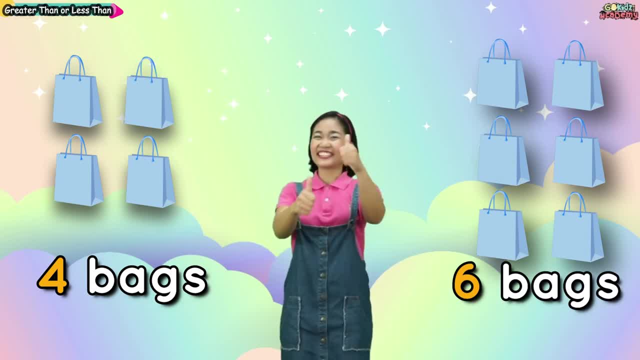 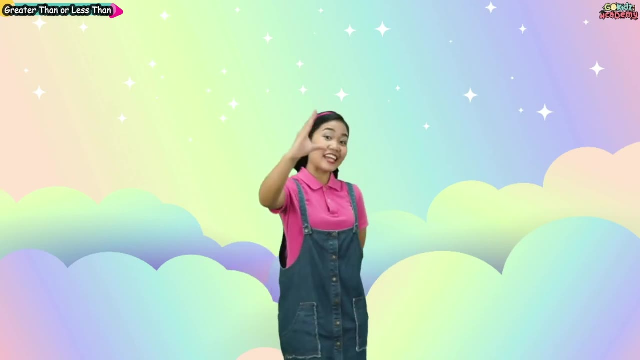 So what's our answer? Very good, Less than Because the number 4 is smaller than the number 6.. Let's have a short activity. Please raise your hand and use this symbol if the number on this side is smaller or less. 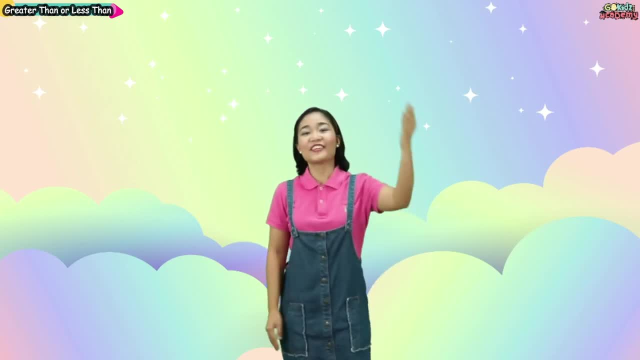 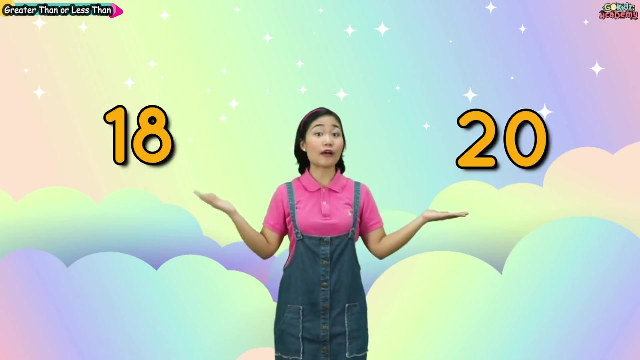 than the number on this side And use this symbol greater than, if the number on this side is bigger than the number 6. Bigger than the number on the other side. Okay, Can you see these numbers? We have 18 and we have 20.. 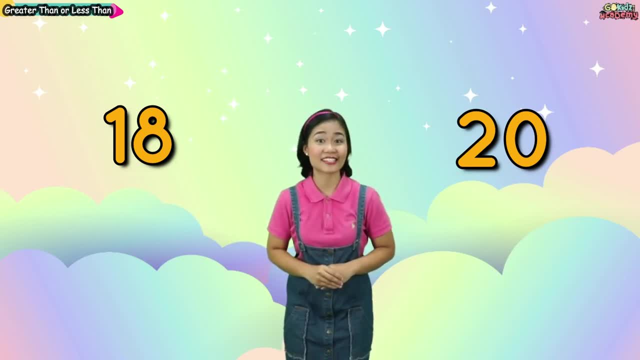 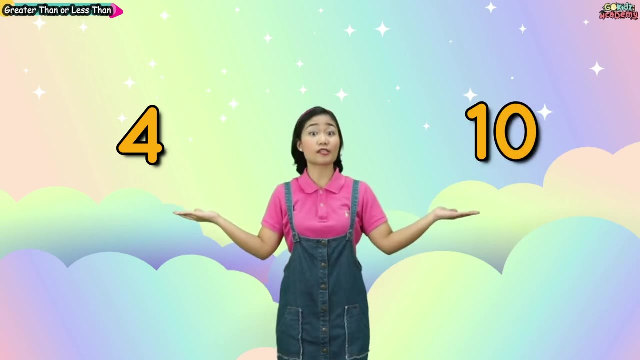 So what symbol should we use? Less than Because 18 is smaller than 20.. We have 4 and we also have 10.. What's our answer? Very good, Less than, again, because 4, of course- is smaller than the number 10.. 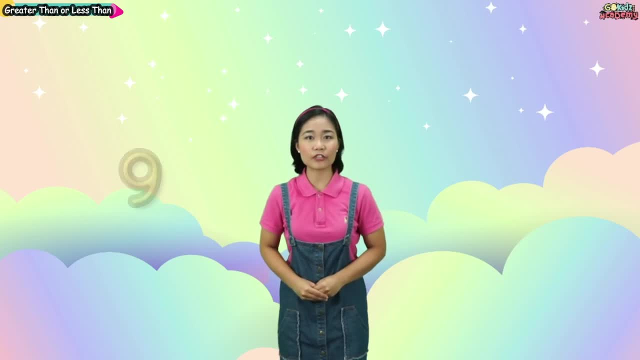 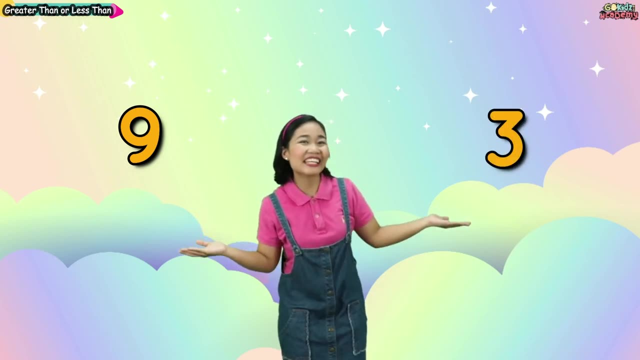 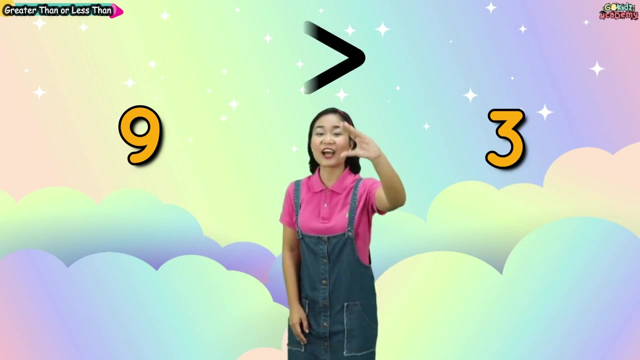 Then let's go to the next. We have here number 9, and what number is this? Number 3.. What symbol should we use? Very good, It's greater than 9,, of course, is bigger than 9.. 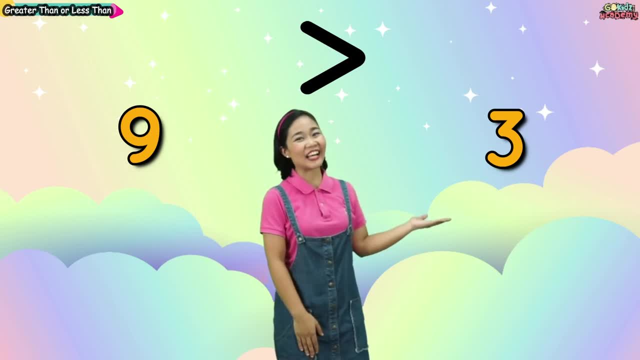 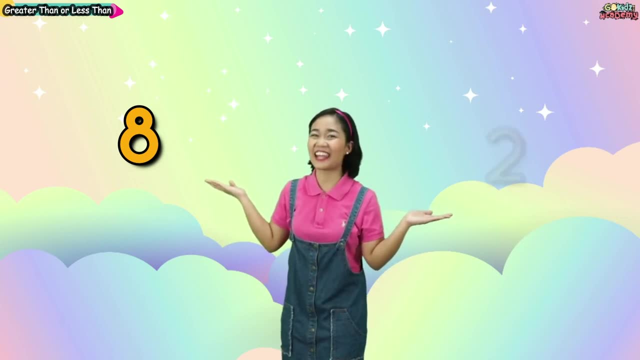 9,, of course, is bigger than 9.. Number 3.. Okay, next numbers. What is this number? again, Very good, Number 8.. And number 2.. What symbol should we use? Very good, The symbol of greater than. 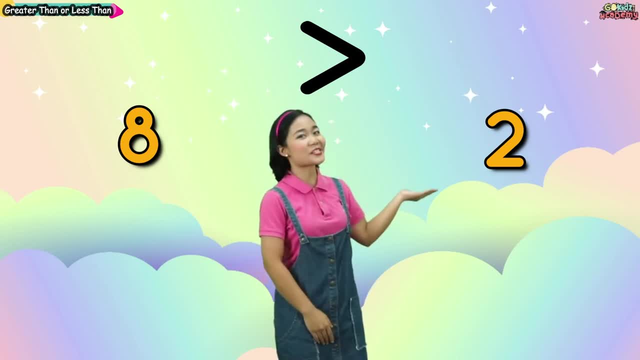 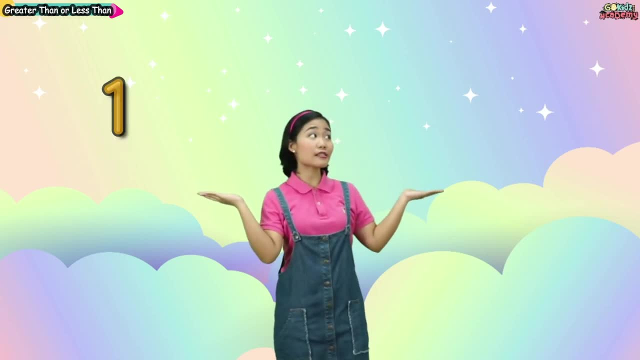 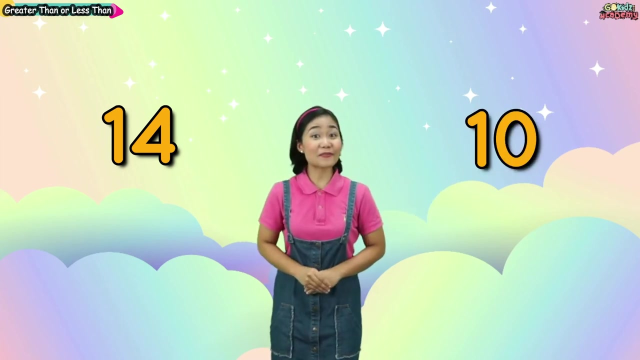 Because 8 is bigger than the number 2.. Oh, This would be the last one for today. What numbers are these? 14 and the number 10.. What symbol should we use? Very good, The symbol of greater than, Because the number 14 is bigger than the number 10.. 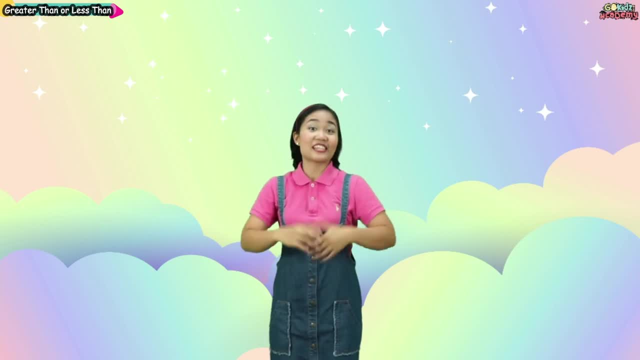 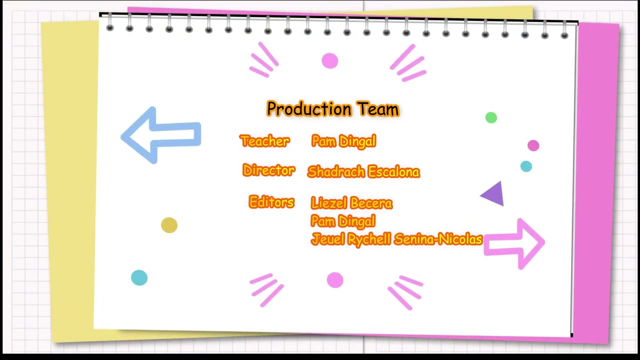 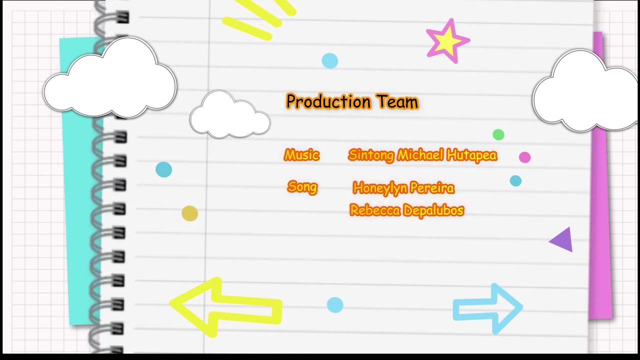 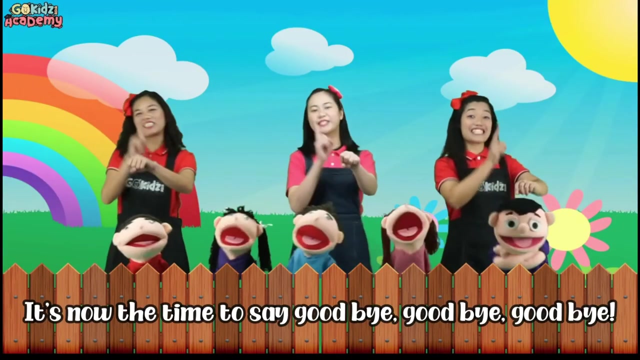 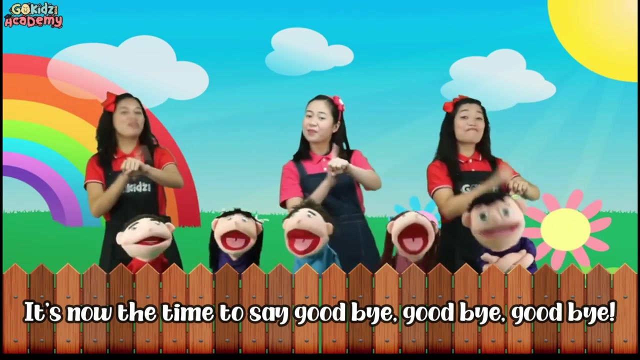 Wow, You did a very good job. That's all for today, kids. I hope you had fun today And I'll see you again on our next video. Bye, Bye. Oh, My luck, We were both wrong, Yay.